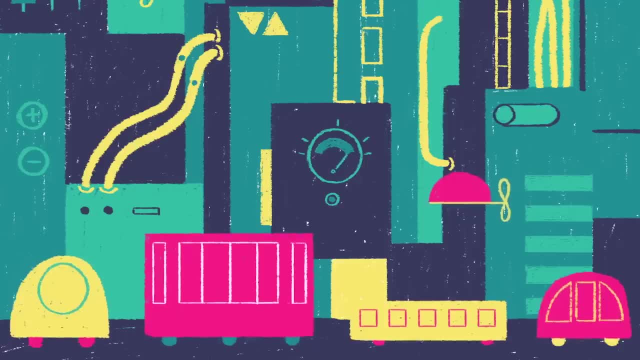 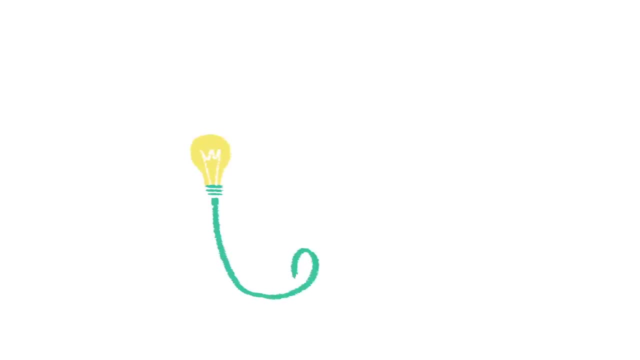 Meanwhile, liquid fuels play a crucial role in almost all forms of transportation. Let's consider the electrical portion first. The great news is that our technology is already advanced enough to capture all that energy from renewables, and there's an ample supply. The sun continuously brings in energy from renewable energy. 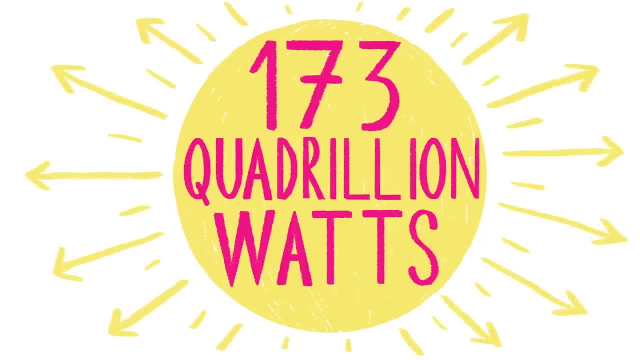 and there's an ample supply. The sun continuously brings in energy from renewable energy and there's an ample supply. Electricity radiates about 173 quadrillion watts of solar energy at the Earth, which is almost 10,000 times our present needs. It's been estimated that a surface that spans several hundred thousand kilometers would be needed to power humanity at our present usage levels. So why don't we build that? Because there are other hurdles in the way, like efficiency and energy transportation, To maximize efficiency. 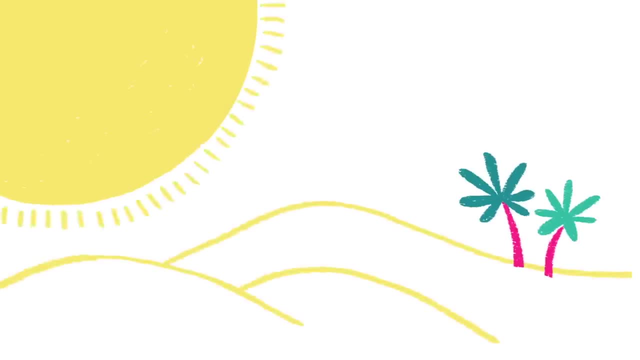 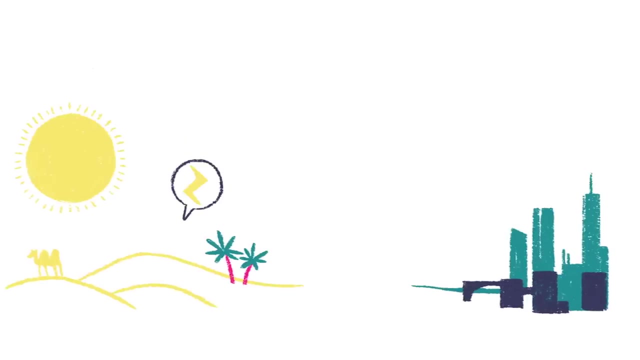 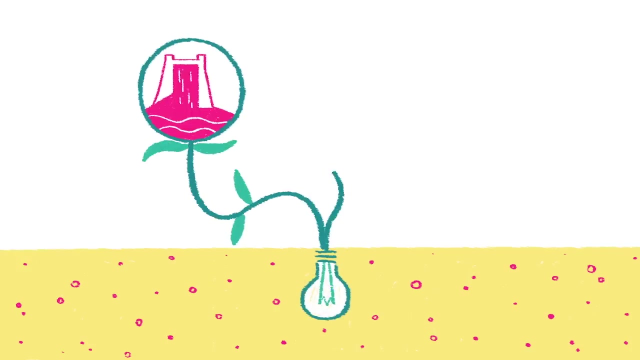 solar plants must be located in energy in areas with lots of sunshine year-round, like deserts, But those are far away from densely populated regions where energy demand is high. There are other forms of renewable energy we could draw from, such as hydroelectric, geothermal and biomasses. 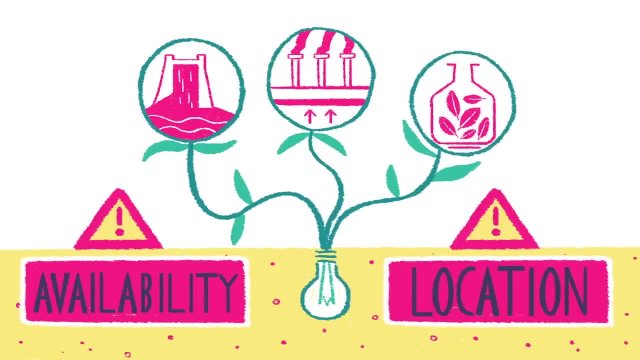 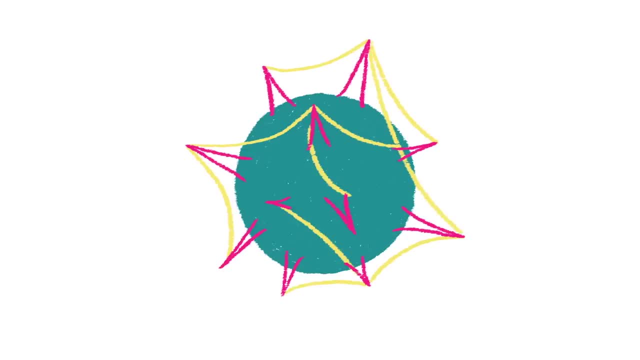 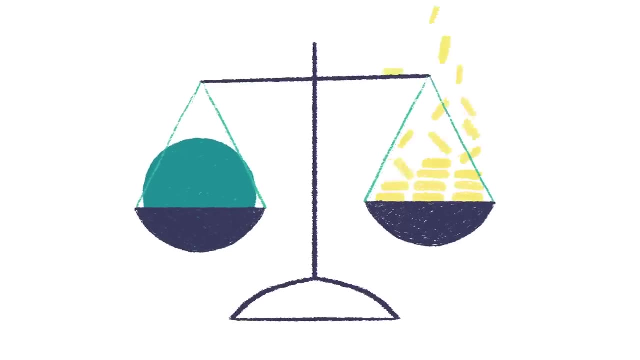 but they also have limits based on availability and location. In principle, a connected electrical energy network with power lines criss-crossing the globe would enable us to transport power from where it's generated to where it's needed, But building a system on this scale faces an astronomical price tag. 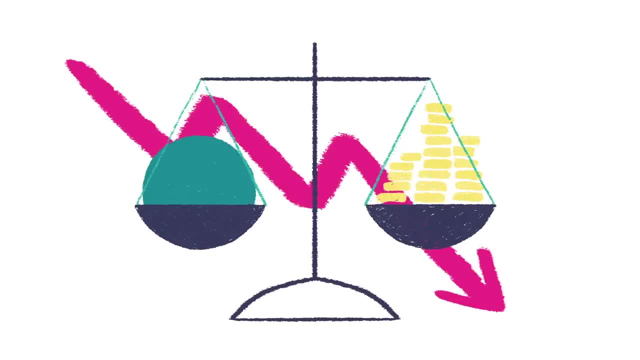 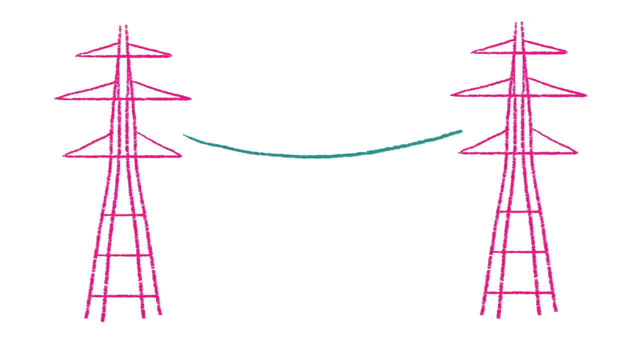 We could lower the cost by developing advanced technologies to capture energy more efficiently. The infrastructure for transporting energy would also have to change drastically. Present-day power lines lose about 6-8% of the energy they carry because wire material dissipates energy through resistance. Longer power lines would mean more energy loss. Superconductors could be one solution. Such materials can transport electricity without dissipation. Unfortunately, they only work if cooled to low temperatures, which requires energy and defeats the purpose To benefit from that technology. 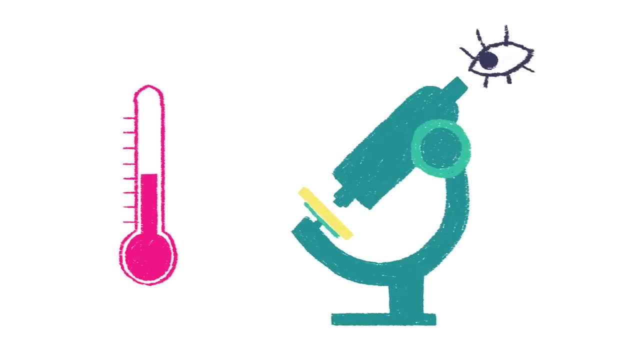 we'd need to discover new superconducting materials that operate at room temperature. And what about the all-important oil-derived liquid fuels? The scientific challenge there is to store renewable energy in an easily transportable form. Recently, we've gotten better at producing lithium-ion batteries. 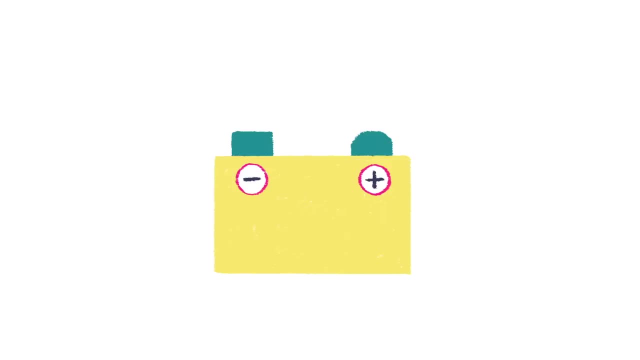 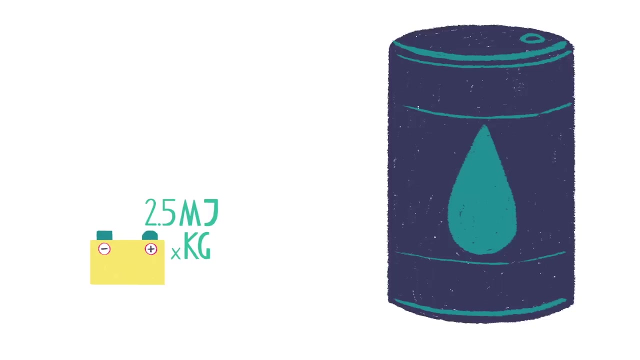 which are lightweight and have high energy density. But even the best of these store about 2.5 megajoules per kilogram. That's about 20 times less than the energy in one kilogram of gasoline, To be truly competitive, car batteries would have to store much more energy without adding cost. The challenge is only interesting if there's an increase for bigger vessels like ships and planes. To power a cross-Atlantic flight for a jet we'd need a battery weighing about 1,000 tons. 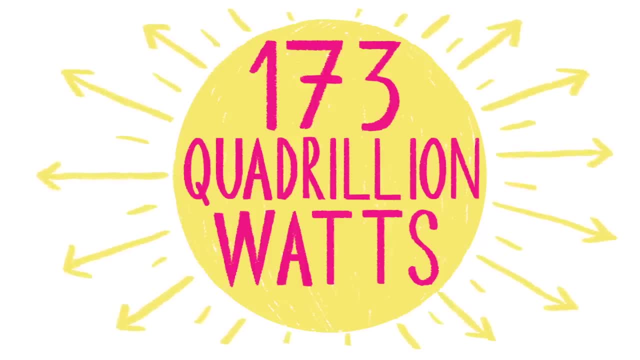 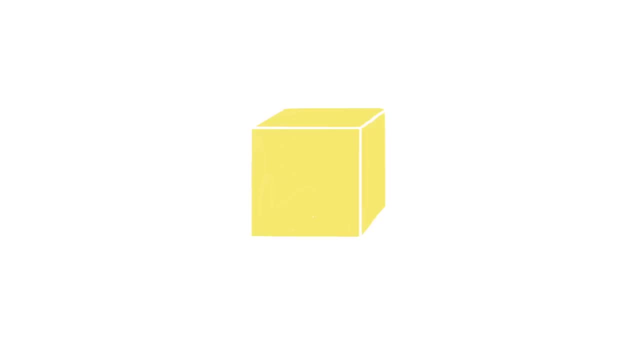 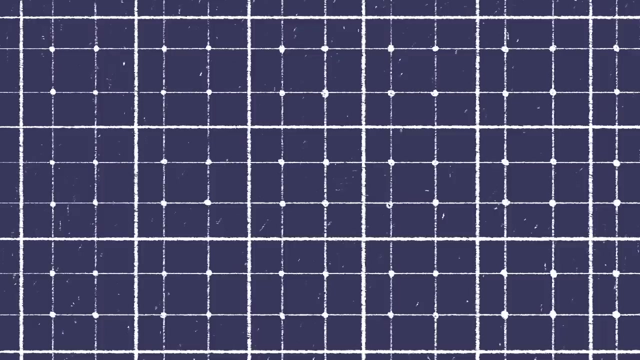 Electricity radiates about 173 quadrillion watts of solar energy at the Earth, which is almost 10,000 times our present needs. It's been estimated that a surface that spans several hundred thousand kilometers would be needed to power humanity at our present usage levels. 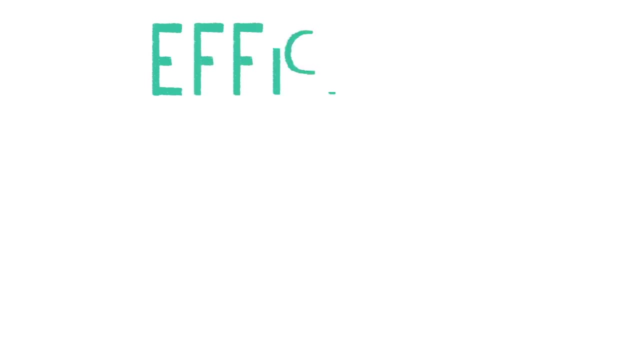 So why don't we build that? Because there are other hurdles in the way, like efficiency and energy transportation. To maximize efficiency, solar plants must be located in areas with lots of sunshine year-round, like deserts, But those are far away from densely populated regions. 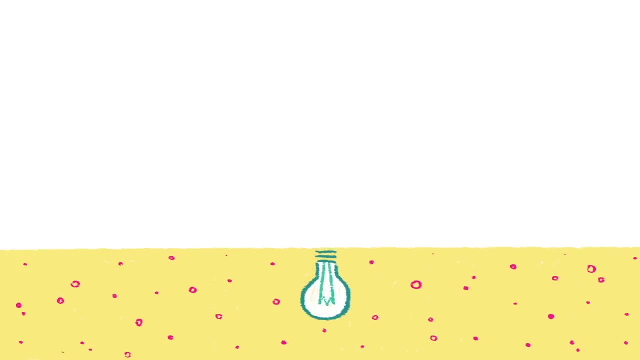 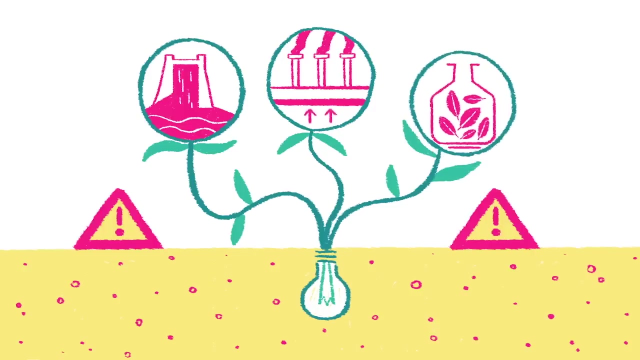 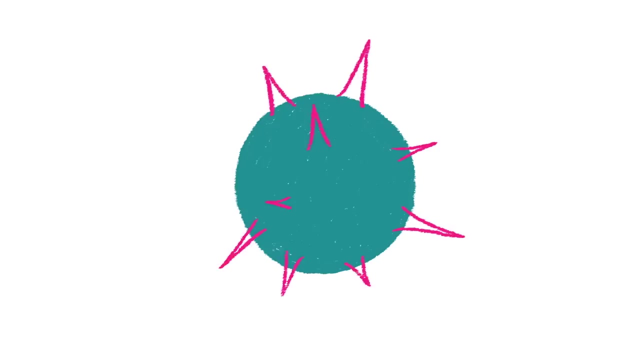 where energy demand is high. There are other forms of renewable energy we could draw from, such as hydroelectric, geothermal and biomasses, but they also have limits based on availability and location. In principle, a connected electrical energy network with power lines criss-crossing the globe. 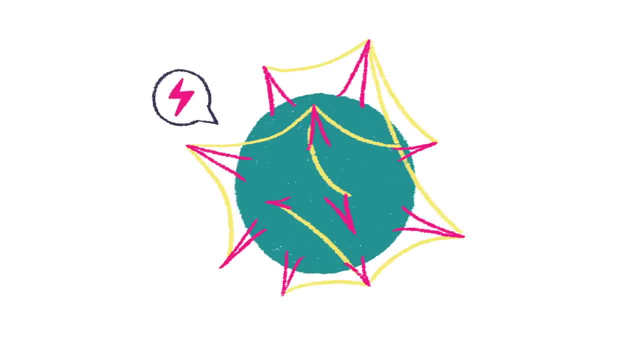 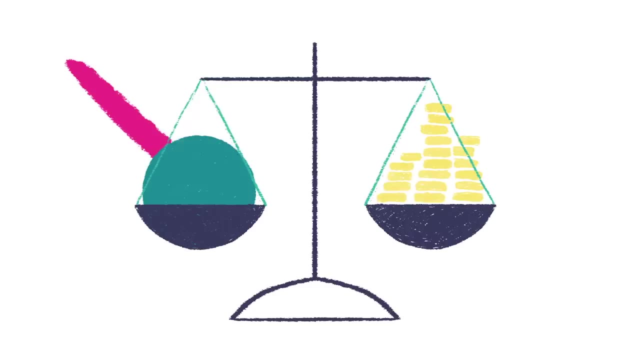 would enable us to transport energy, would enable us to transport energy. would enable us to transport energy from where it's generated to where it's needed. But building a system on this scale faces an astronomical price tag. We could lower the cost by developing advanced technologies. 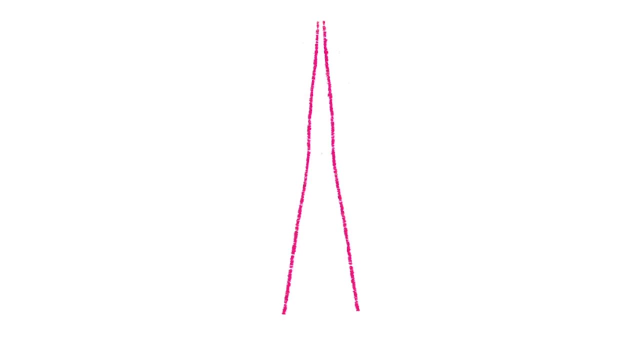 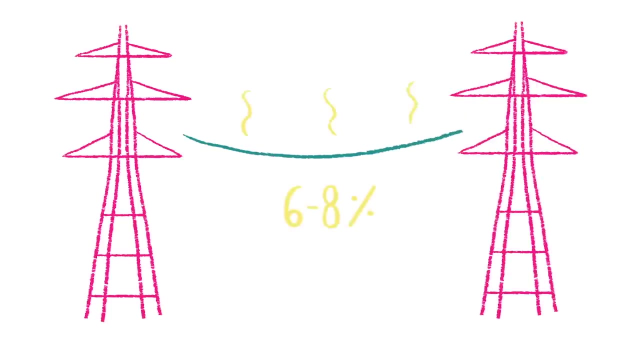 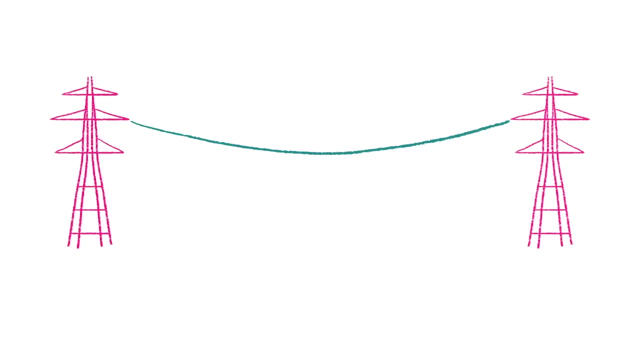 to capture energy more efficiently, The infrastructure for transporting energy would also have to change drastically. Present-day power lines lose about 6 to 8% of the energy they carry because wire material dissipates energy through resistance. Longer power lines would mean more energy loss. 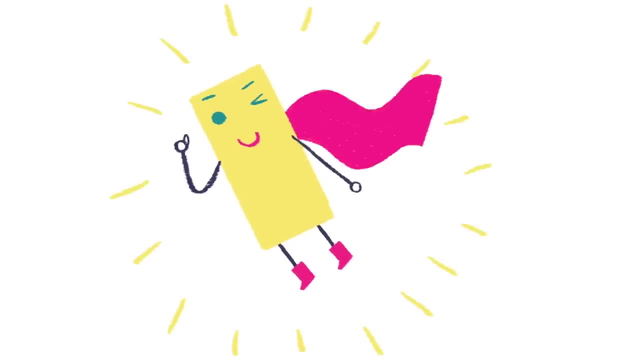 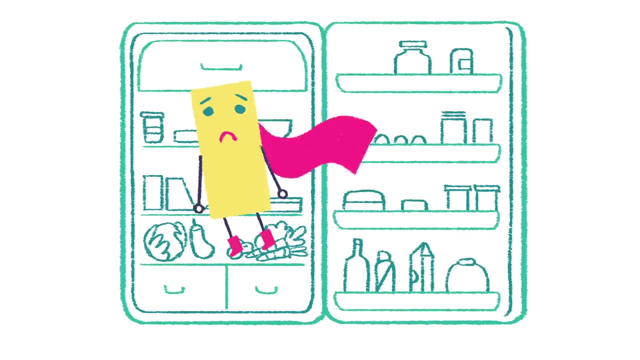 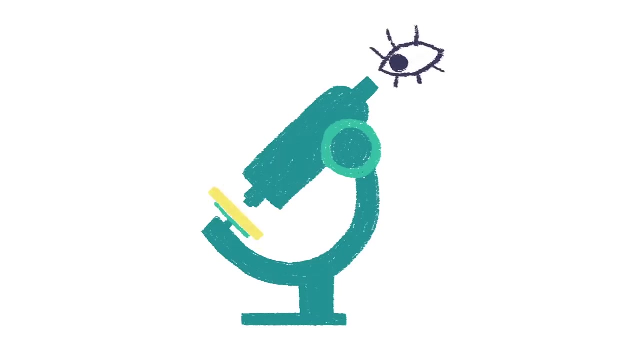 Superconductors could be one solution. Such materials can transport electricity without dissipation. Unfortunately, they only work if cooled to low temperatures, which requires energy and defeats the purpose. To benefit from that technology, we'd need to discover new superconducting materials. 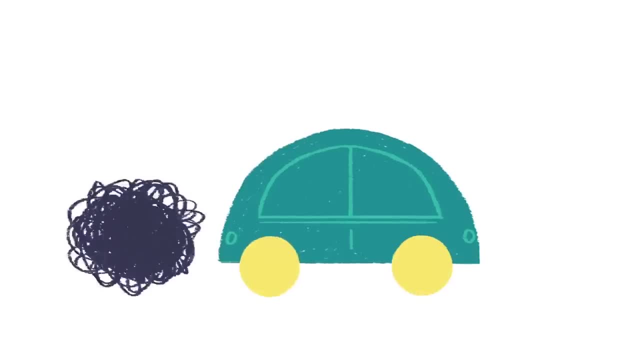 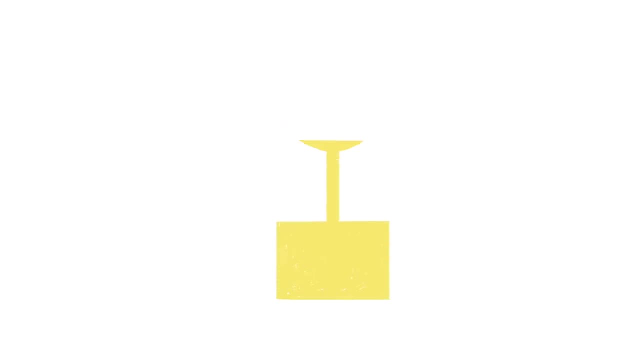 that operate at room temperature? And what about the all-important oil-derived liquid fuels? The scientific challenge there is to store renewable energy in an easily transportable form. Recently, we've gotten better at producing lithium-ion batteries, which are lightweight and have high energy density. 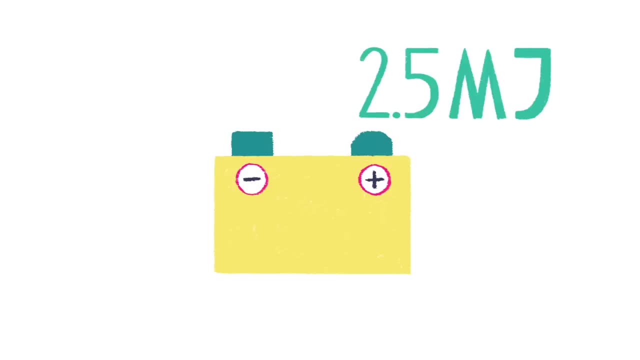 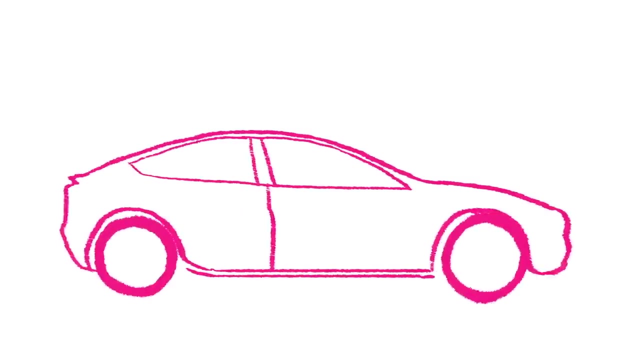 But even the best of these store about 2.5 megajoules per kilogram. That's about 20 times less than the energy in one kilogram of gasoline. To be truly competitive, car batteries would have to store much more energy without adding cost.